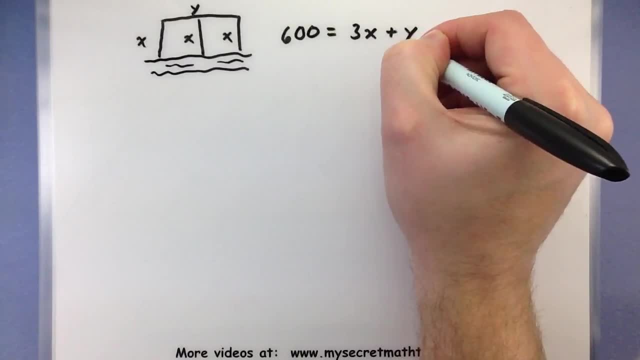 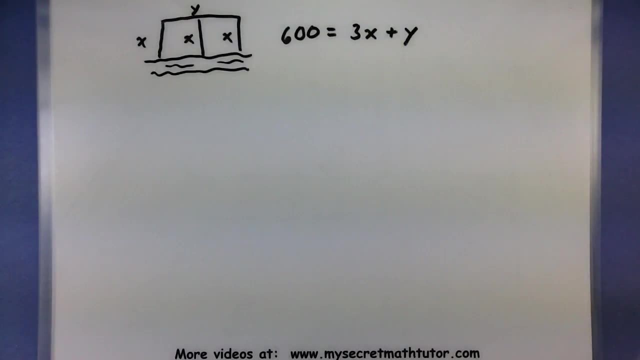 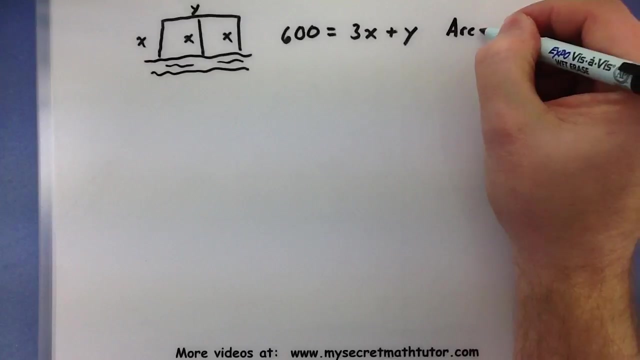 So I have three of my short pieces, or 3x, plus one long piece, y. Hmm, now, by itself that does not look quadratic. Well, I also want to keep in mind that I'm looking for the maximum area, So the area of this shape would be equal to the maximum area. 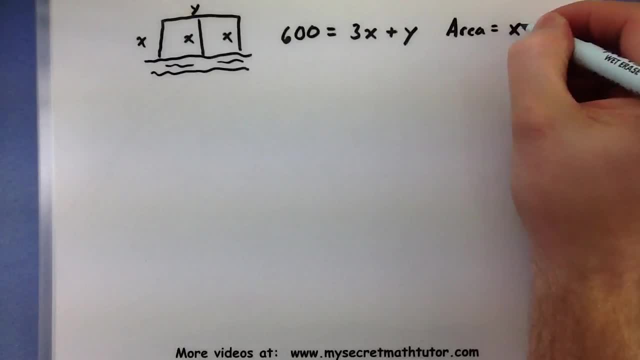 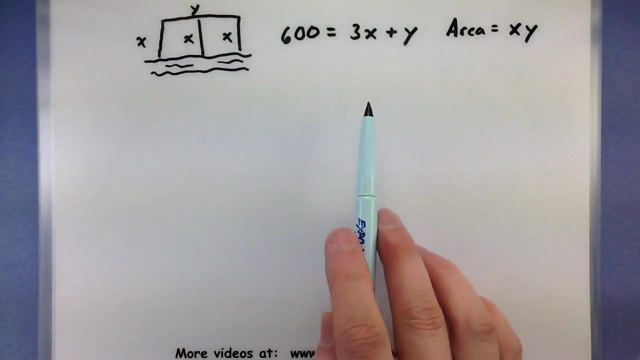 equal the width and the length multiplied together, or x times y. Now, if I can put these two things together, I can actually form a quadratic. Here's the idea. I have an x times y over here and I have some x's and y's over here. We're going to solve this. 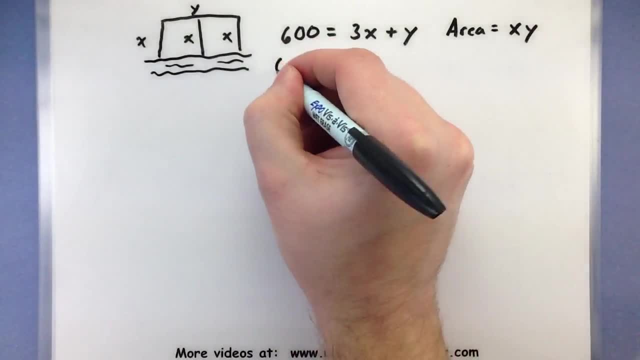 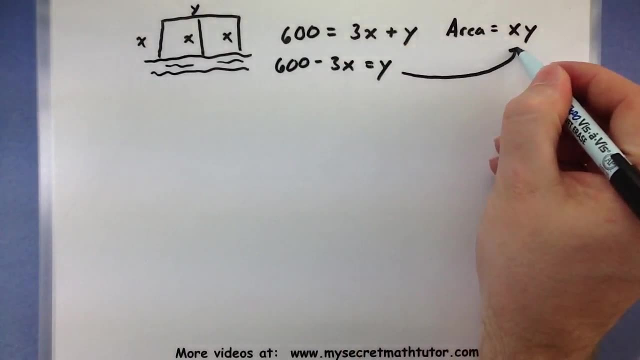 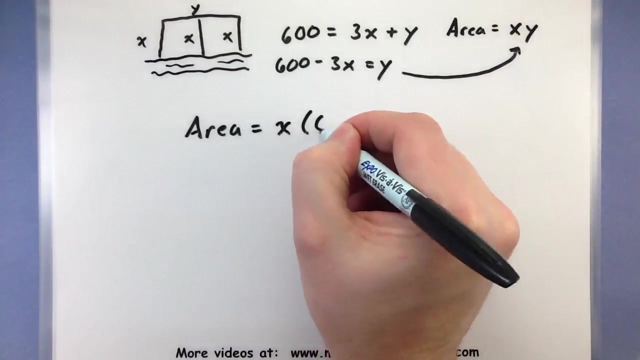 one for y and put it into the area. So 600 minus 3x is equal to y. We'll go ahead and put it right in there for y. So area is equal to x multiplied by 600 minus 3x. There we. 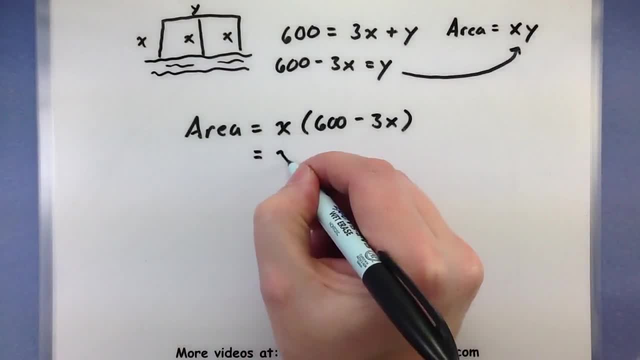 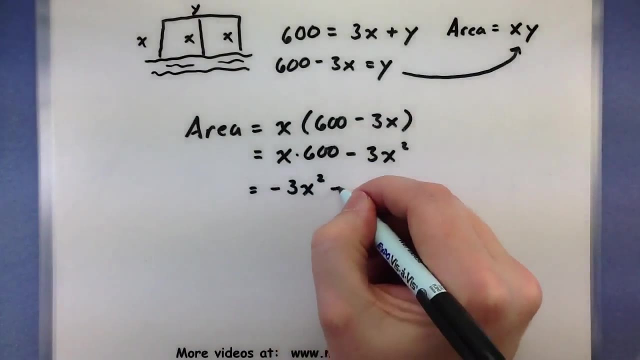 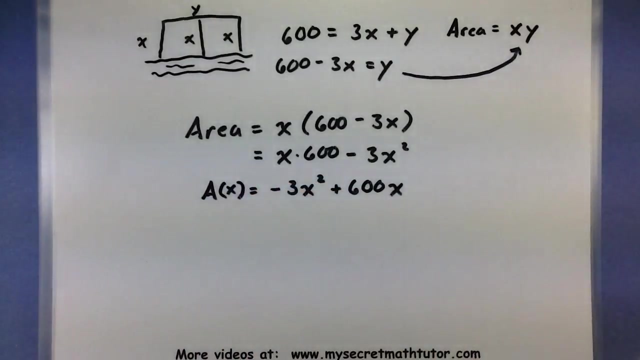 go Now. continuing to multiply through, I get x times 600 minus 3x squared. Let's go ahead and rearrange the terms so that our power is from largest to smallest. So negative 3x squared Plus 600x. All right, So from my given conditions, I've set up a quadratic function here Now. 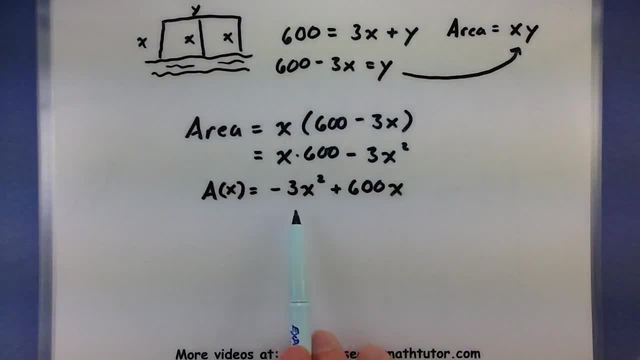 what we want to do is figure out where's the maximum area or where's the maximum of this quadratic function. So we'll use x equals negative b, all over 2a to find out Our values that we'll pick out for this. 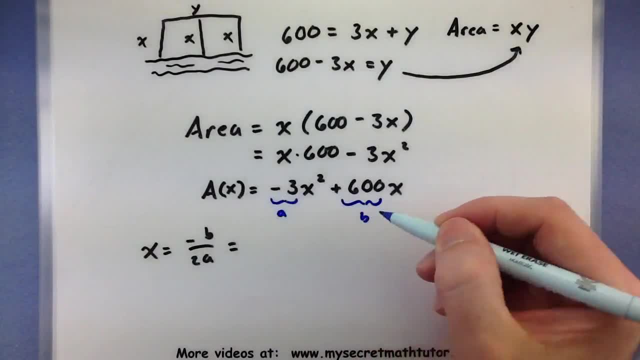 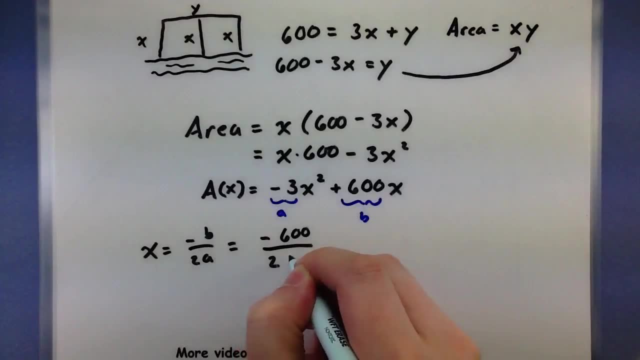 The negative 3 will be the a and the 600 will be the b. So I have negative 600 all over 2 times the negative 3.. So 600 negative divided by negative 6, or 100.. So since I'm 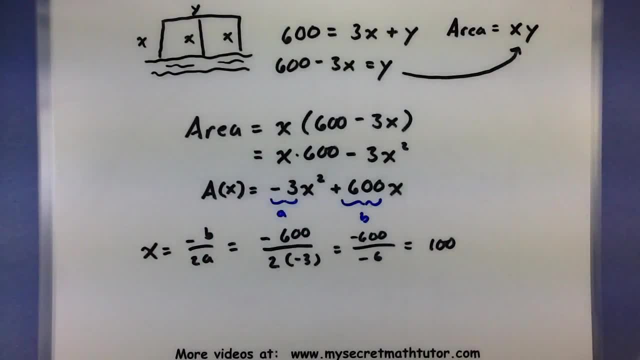 using x for the lengths of my small sides, and it equals 100,. it tells me that our fencing so far is going to be negative 3.. So I'm going to use x for the lengths of my small sides, and it equals 100.. So, since I'm using x for the lengths of my small sides and it equals.